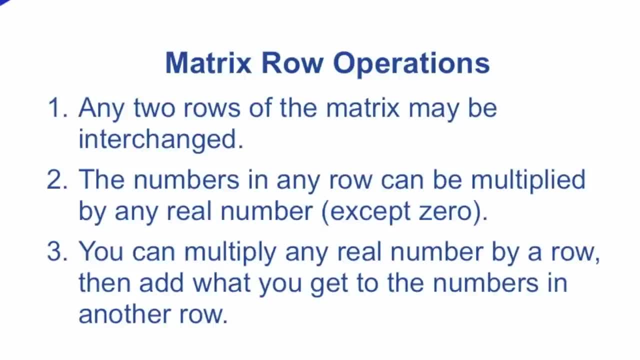 First, any two rows of the matrix can be interchanged. They can switch places. Second, the numbers in any row can be multiplied by any real number except for zero. And third, we can multiply any real number by a row, then add what we get to the numbers in another row. 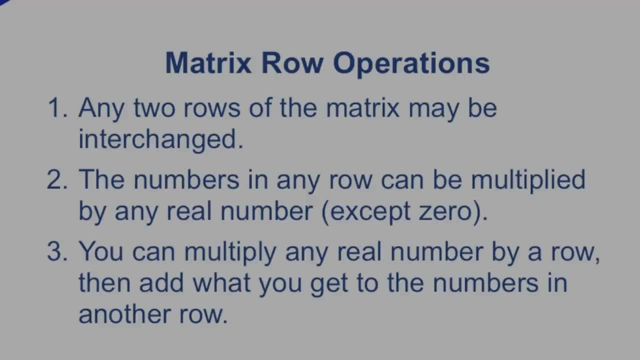 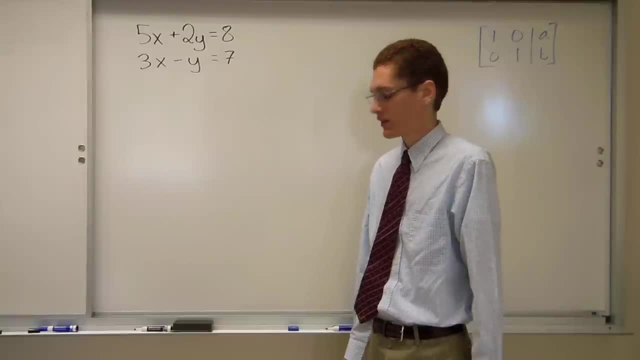 This will make more sense once we see an example. I have the system of equations: 5x plus 2y equals 8, and 3x minus y equals 7.. First I'll have to put that into an augmented matrix. 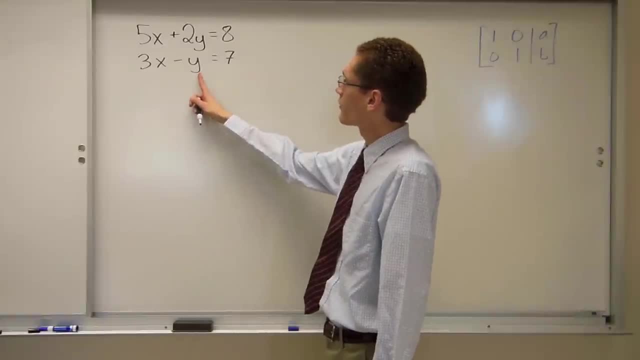 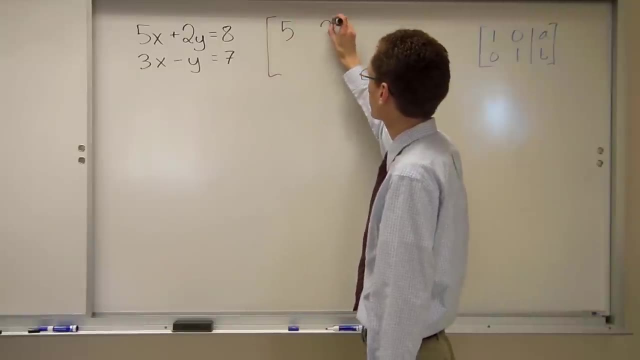 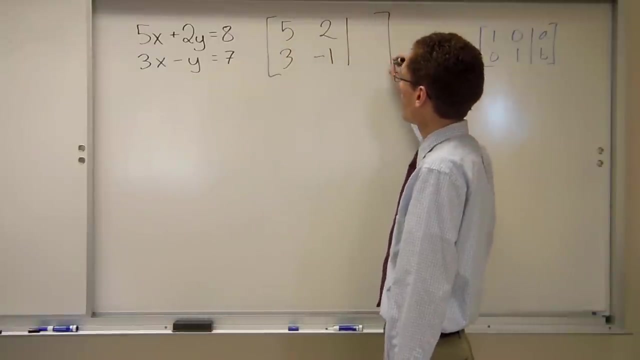 I do this by adding a matrix. I do that by lining up the x terms, the y terms and the constants and just taking the coefficients, In this case 5,, 2,, 3, and it's like there's a negative 1 times that y. 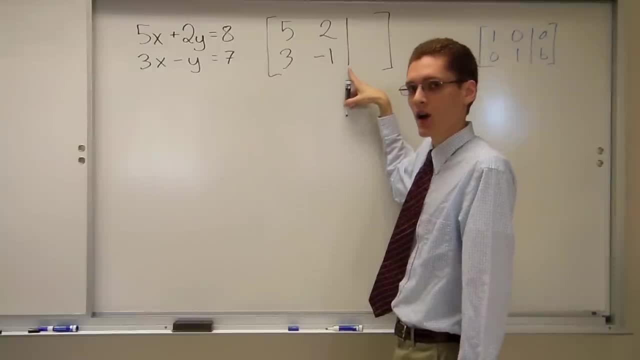 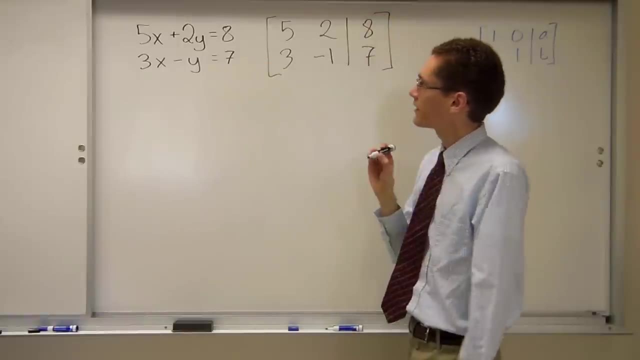 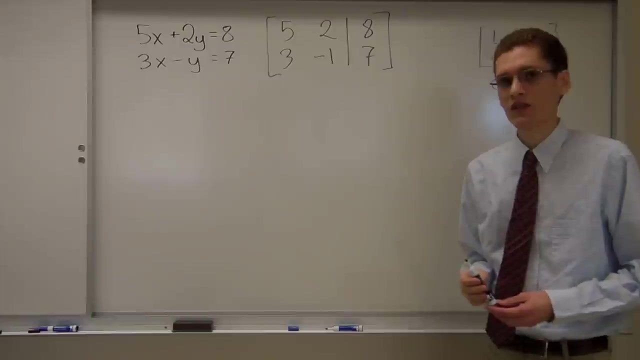 And then drawing this line, which is what makes it an augmented matrix, and that lines up with the equals signs. Then I have 8 and 7. So I've created an augmented matrix using this system of equations. My next step is to use the matrix row operations to get the matrix into row echelon form. 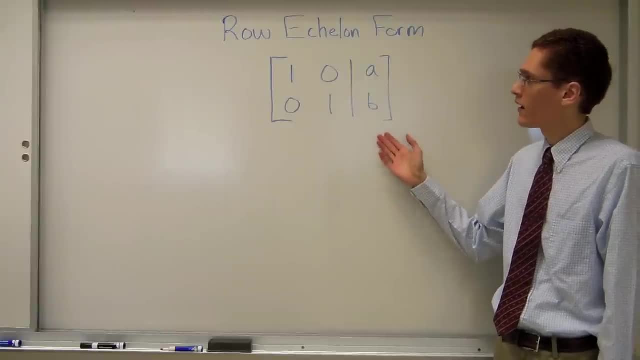 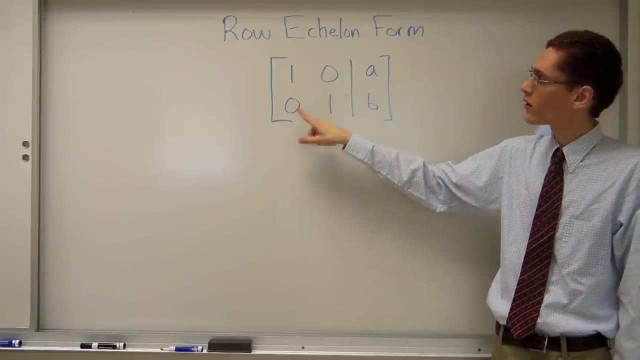 which for a 2x3 matrix looks like this: In the first row, in the first column, we have a 1.. First row, second column, a: 0.. Second row, first column, a 0.. And second row, second column, a 1.. 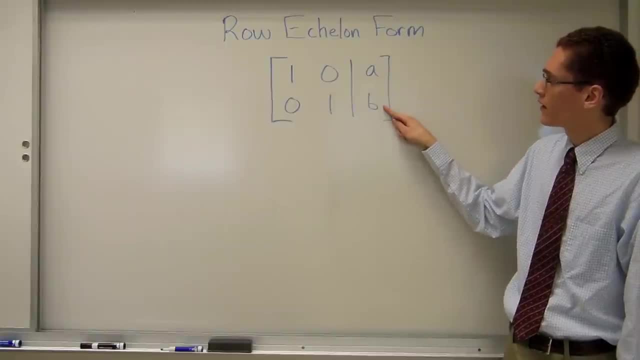 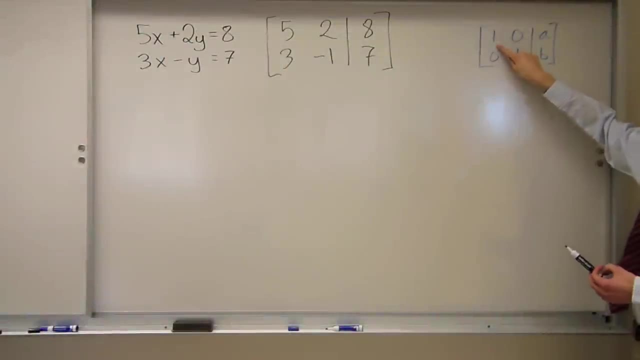 And then the numbers on the other side of the line which represents the equals sign can be anything. I'm going to start with trying to get the 5 to be 1 in this first place here. Now I know I can multiply by any number other than 0.. 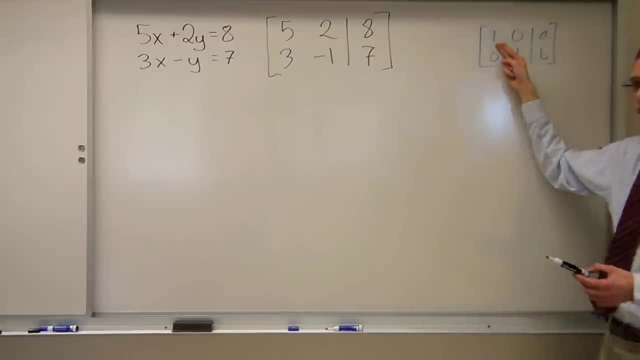 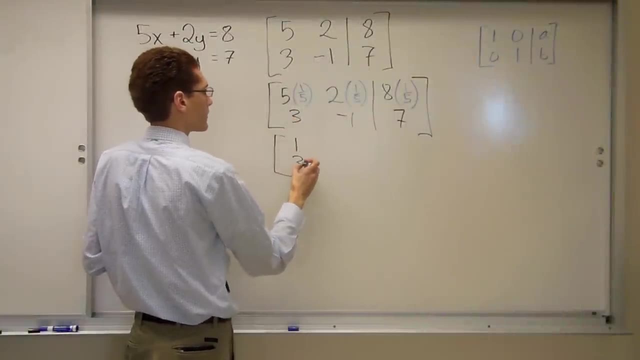 So if I multiply 5 by 1 fifth, I can get it to be 1.. So I'll do that. So when I multiply those out 5 times 1 fifth is 1.. 2 times 1 fifth. we'll just write 2 fifths. 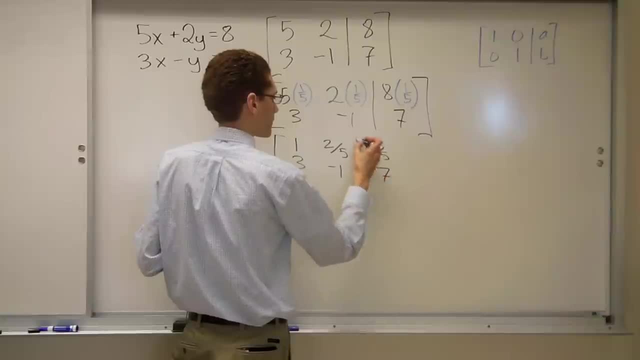 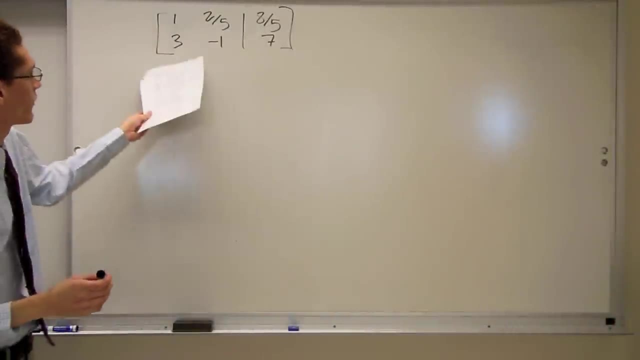 8 times 1 fifth, we'll have to write 8 fifths. So I have this augmented matrix. So I've copied my matrix again over here. Now I'm going to use the third matrix row operation to get the 3 to be a 0.. 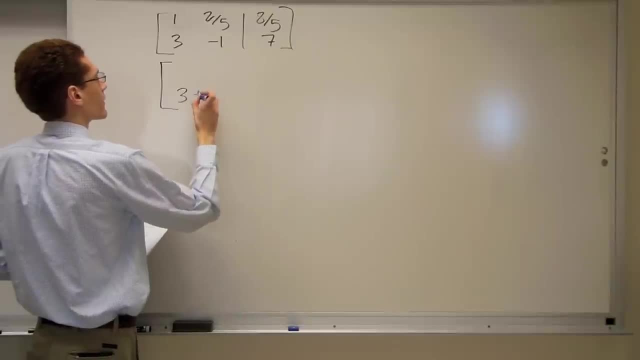 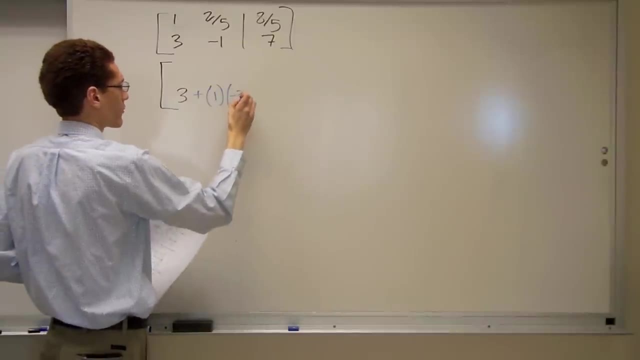 I'm going to take the 3, and I'm going to add to it the number from the row above 1, times any real number. In this case, negative 3 is what will work, because 3 plus 1 times negative 3 is going to be 0,. 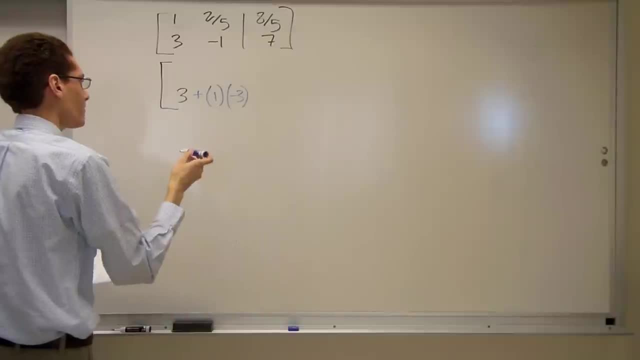 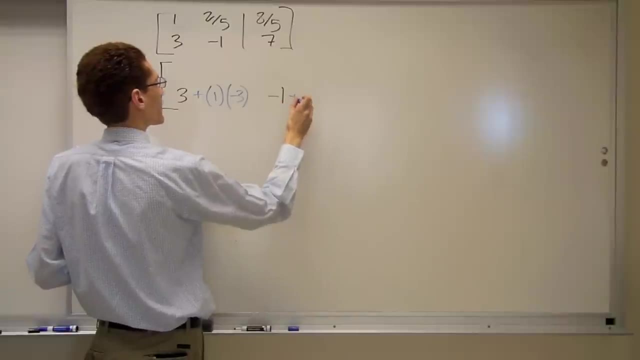 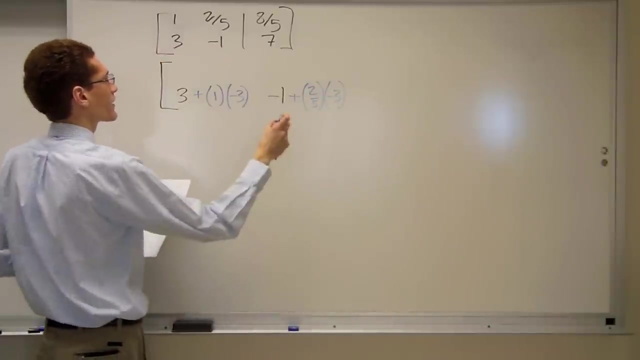 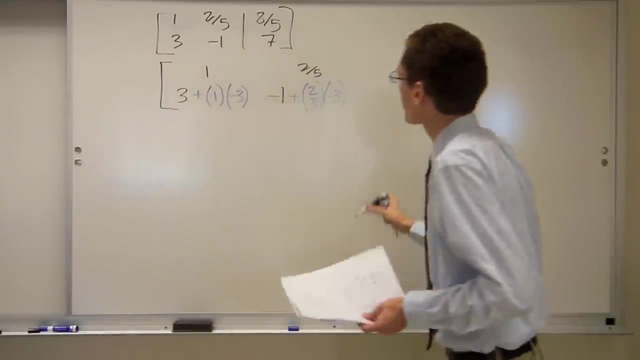 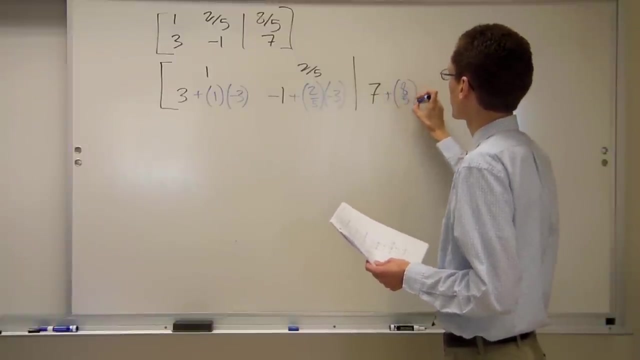 which is what I'm aiming for. So I'll do that with the next terms as well. We have negative 1 plus 2 fifths times negative 3.. Again, the 2 fifths came from the line above. And then I have 7 plus 8 fifths times negative 3.. 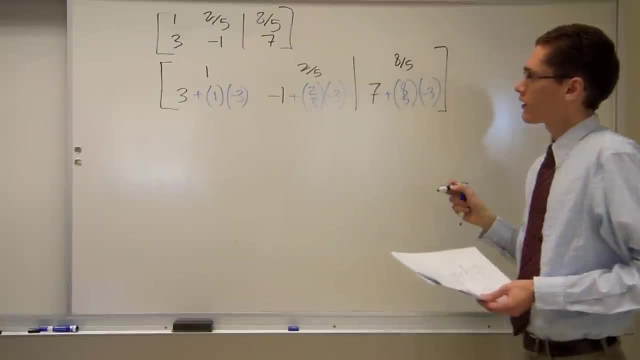 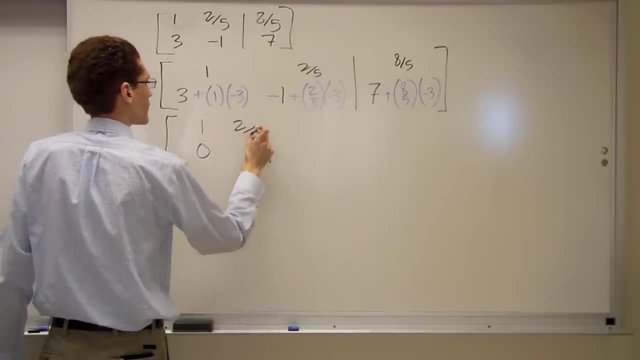 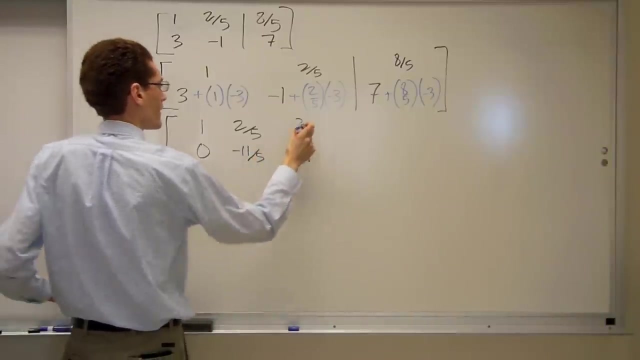 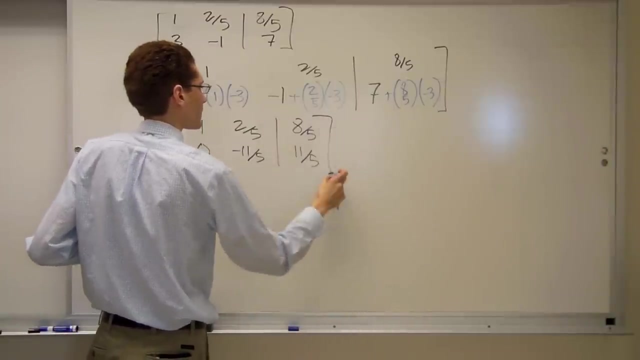 I still have an 8 fifths up here, So this one simplifies to 1,, 0,, 2 fifths, negative 11 fifths, 8 fifths and positive 11 fifths. Now we still need that 2 fifths to be a 0,. 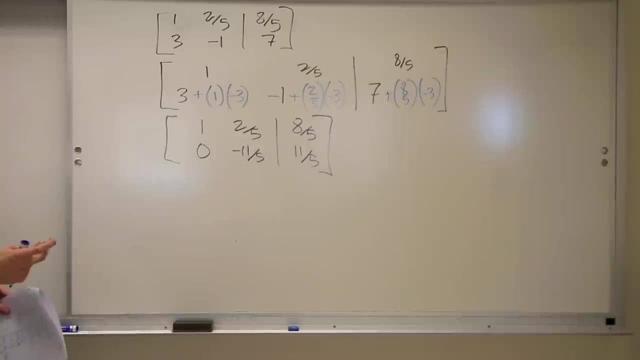 and that negative 11 fifths to be a 1.. I'll start with the negative 11 fifths. To cancel out the negative 11 fifths and make it positive 1, I'll multiply by negative 5 elevenths. 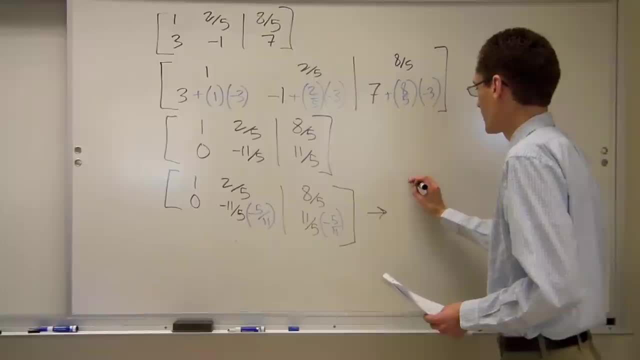 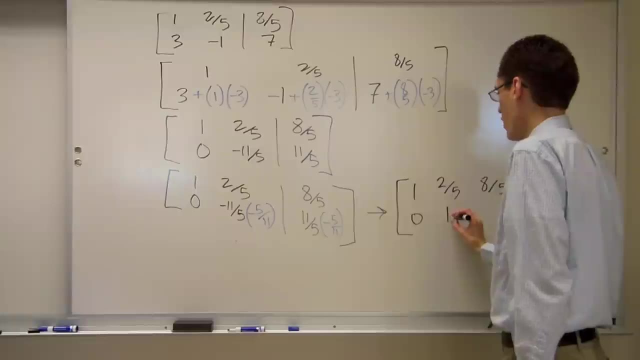 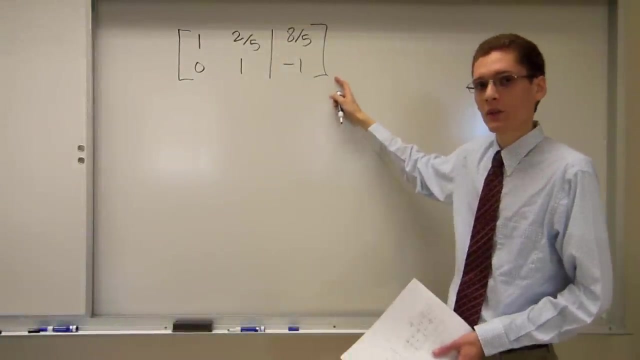 So that's going to be the matrix: 1, 2 fifths, 8 fifths 0, 1, negative 1.. So we have this matrix and we're still not quite yet in row H1 form, because that 2 fifths should be a 0..